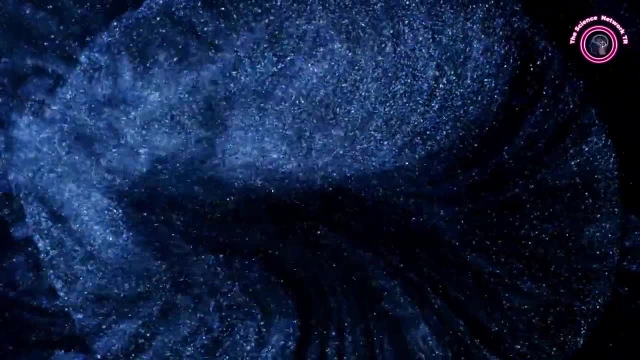 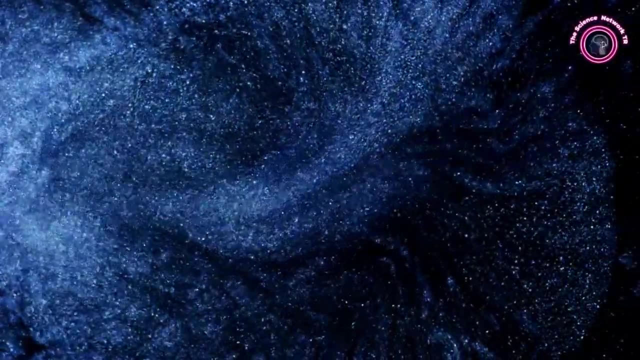 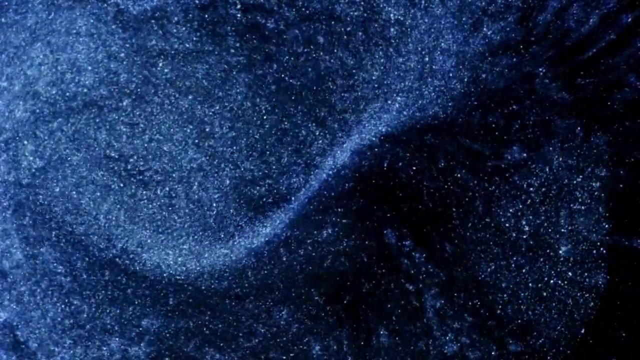 High-energy astrophysics has made great strides in understanding the origins and physics behind these explosive phenomena. Active galactic nuclei exhibit strong emissions across the electromagnetic spectrum. High-energy observations have revealed the existence of supermassive black holes and their role in shaping galactic evolution. The remnants of supernova explosions. 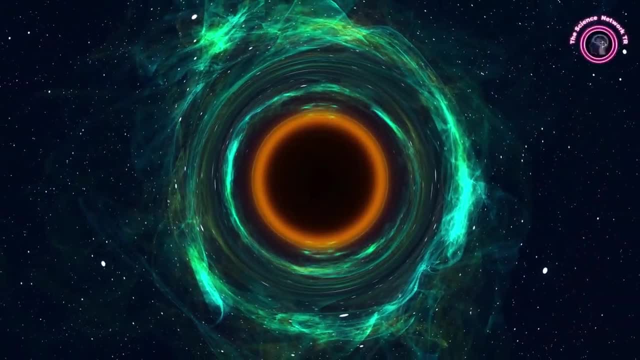 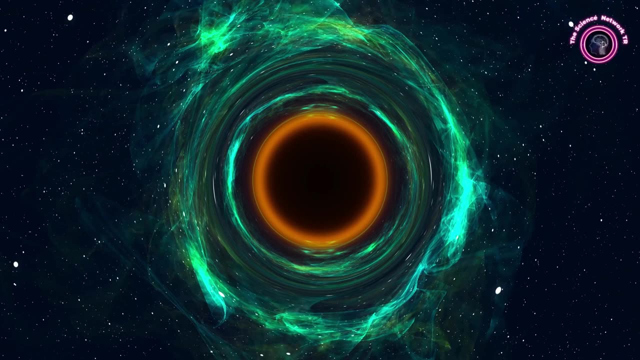 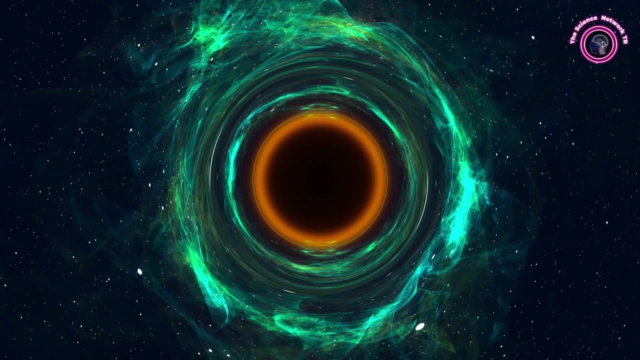 emit high-energy energy from the galaxy, High-energy radiation that provides information about stellar evolution, nucleosynthesis and the distribution of cosmic rays. By studying cosmic rays and high-energy particles, scientists better understand their origin and the processes responsible for their acceleration in astrophysical sources. Ongoing research in high-energy astrophysics continues. 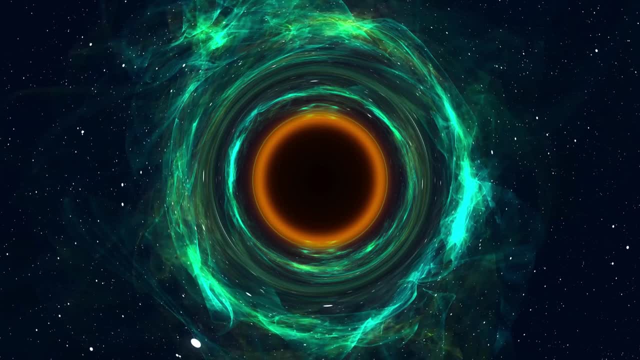 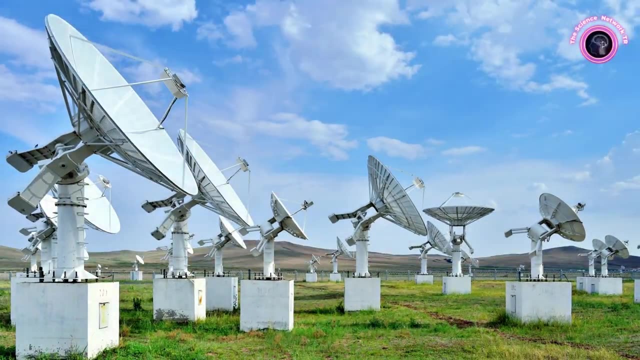 to push the boundaries of our knowledge. Scientists are developing advanced observatories such as the Cherenkov Observatory and the Cherenkov Observatory and the Cherenkov Observatory and the Cherenkov Telescope Array and the James Webb Space Telescope, to explore the universe in even 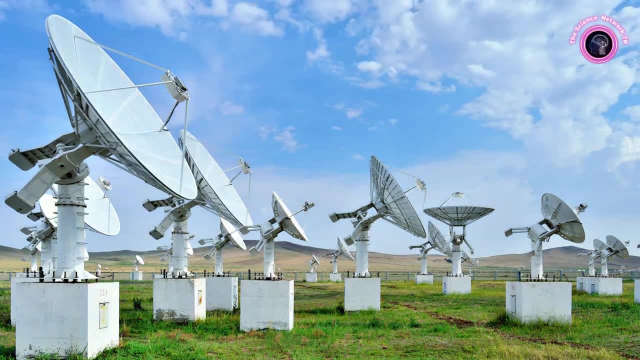 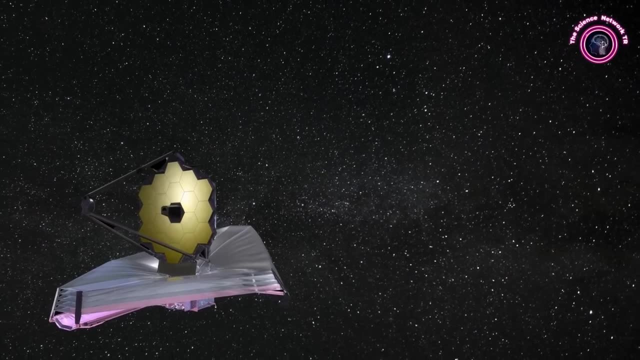 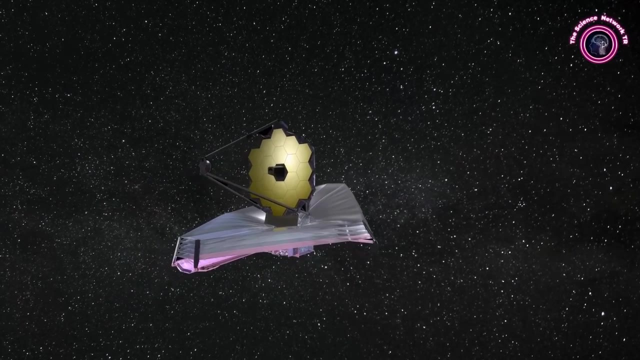 greater detail. Efforts focus on investigating the enigmatic nature of dark matter, understanding the dynamics of cosmic particle acceleration and exploring the early universe through high-energy observations. High-energy astrophysics offers us a fascinating window into the most energetic and extreme phenomena in the universe. Scientists have made remarkable discoveries. 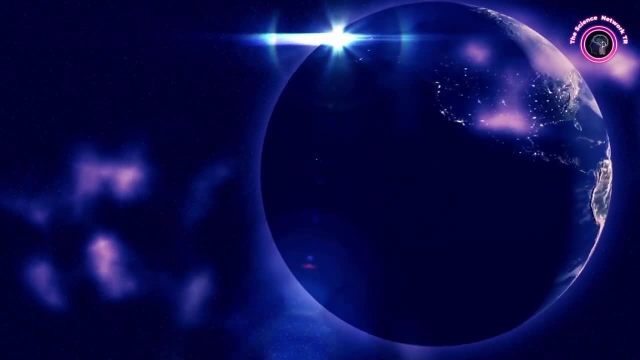 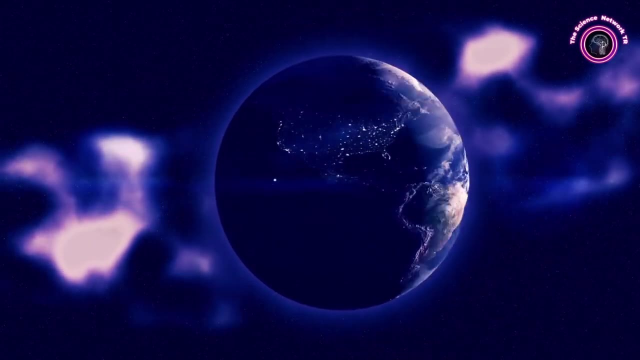 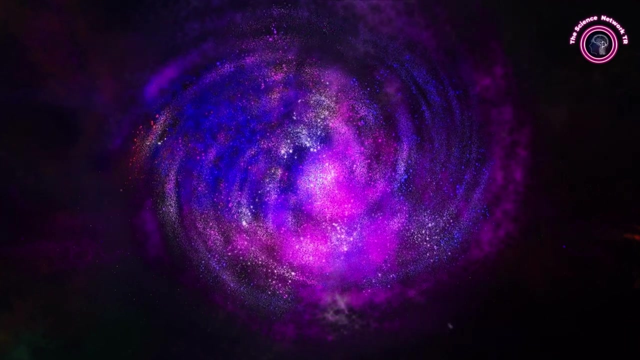 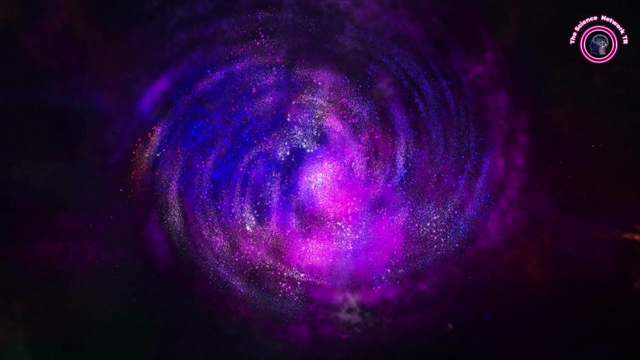 by studying celestial bodies that emit X-rays and gamma rays, expanding our understanding of black holes, galaxy evolution and the fundamental nature of the cosmos. As technology advances and new observatories open, the future of high-energy astrophysics holds the promise of unlocking even more cosmic wonders and deepening our appreciation for the awe-inspiring 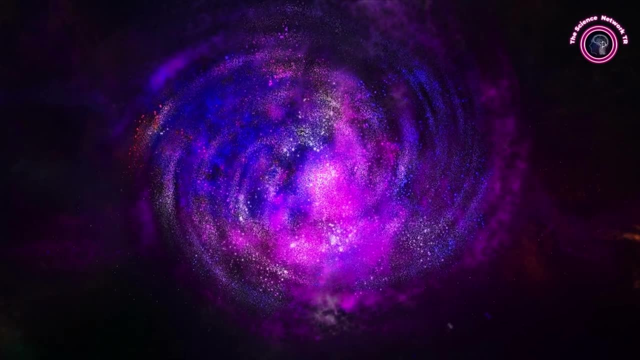 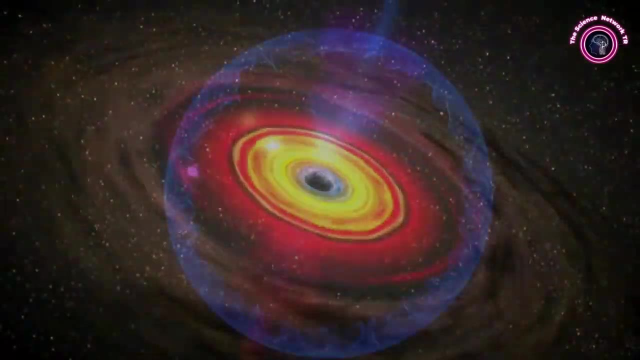 universe we live in. Thank you for joining us on this exciting journey into the fascinating field of astrophysics. In the next video we will continue to think about the formation, types and properties of black holes. See you later.